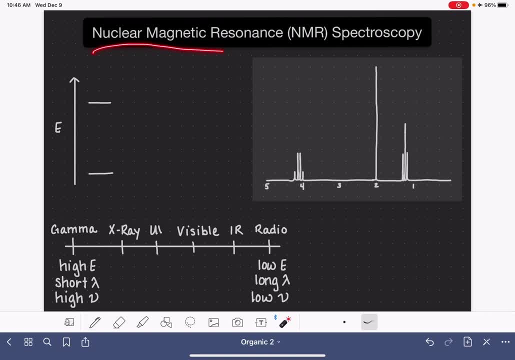 This video is going to be a very brief and basic introduction to the theory of NMR or nuclear magnetic resonance spectroscopy. NMR spectroscopy involves interaction between radio frequency, so that's energy that corresponds to the radio portion of the electromagnetic radiation spectrum, interaction between radio frequency and the nuclei of our atoms, So over. 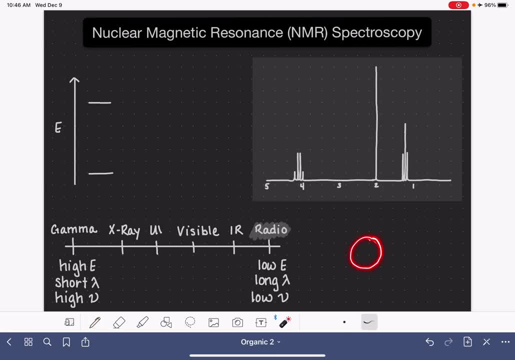 here I'm drawing a nucleus. I'm just modeling the nucleus as a sphere. In general chemistry, when you learn about quantum numbers- N L, M sub L and M sub S- you learn that the nuclei in atoms are constantly spinning on their own axis. You learn about this with the M sub S quantum. 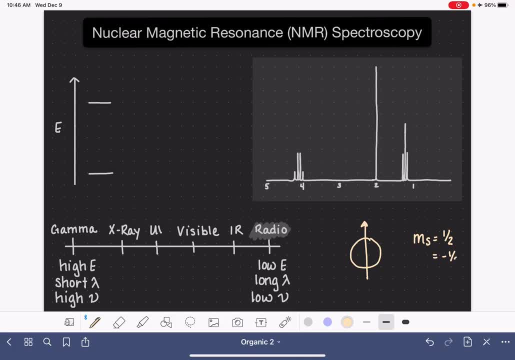 number which we learn has the values, potential values, of one half or minus one half, corresponding to a clockwise spin or a counterclockwise spin. Again, we're referring to the spinning of the nucleus on its own axis, Because the nucleus is a charged particle- remember- it contains a lot of. 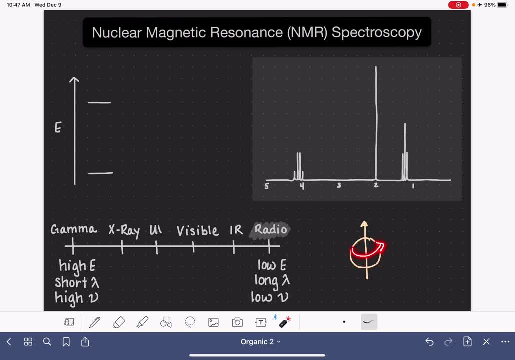 protons which are positively charged. as this nuclei spins- clockwise or counterclockwise- on its own axis, it generates its own little magnetic field, And this is going to be important when we're talking about NMR. So when we want to obtain an NMR spectrum for a molecule, we take our 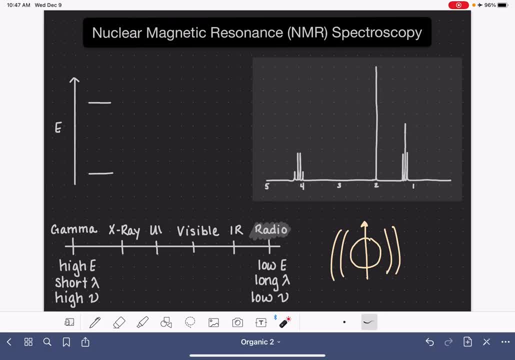 molecule, we put it into the instrument and then we subject the molecule to the instrument. And then we subject the molecules to a very strong external magnetic field, Because our nuclei are like little, teeny, tiny magnets. as they're spinning on their axis they're generating their own little 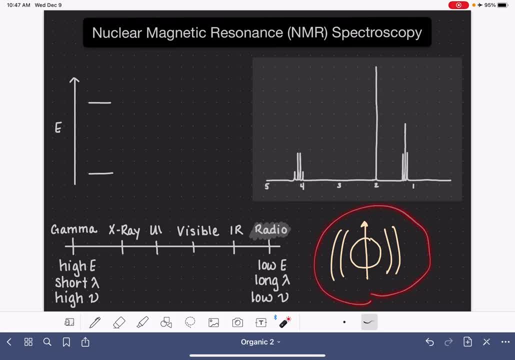 magnetic field. When we drop all of these molecules into a magnetic field, the molecules interact with and align with the magnetic field of the NMR instrument. So this causes all of our little nuclei to align with the NMR's magnet And I'm just going to kind of model that in this NMR. 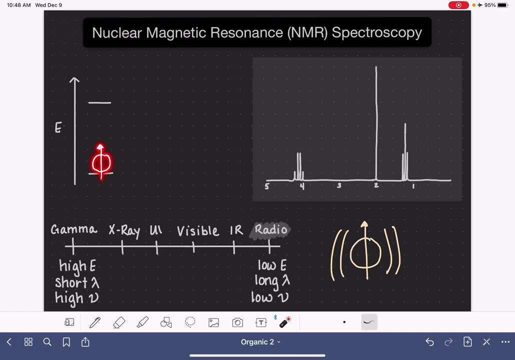 Here's my little energy diagram over here. Here's my little nucleus, Here's its little axis of rotation. It's in a low energy configuration and it is aligned with the NMR's magnet. So once we get all of our nuclei aligned with the NMR magnet, we then take some radio frequency and we blast all of these.